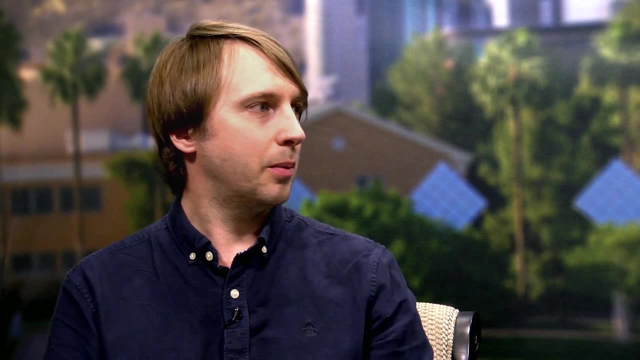 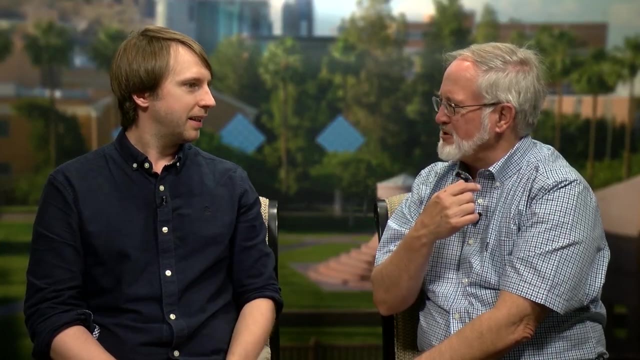 Oh, so I mean, a good example would be making an enzyme. If you release an enzyme into the environment, it breaks down some kind of foodstuff that you can't eat normally, Or the back of your throat for a streptococcus perhaps. 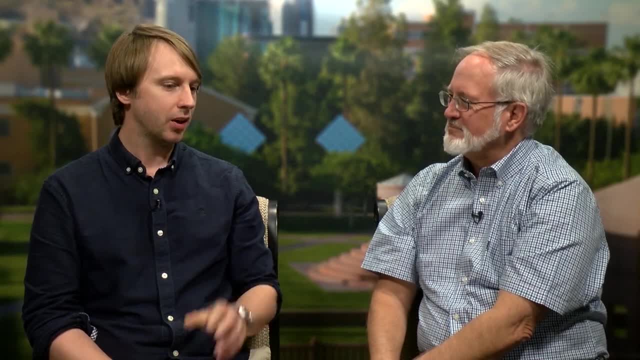 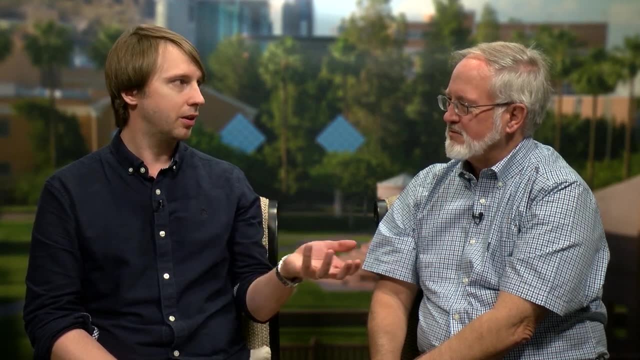 Yeah, yeah, it could also be there, unfortunately, That's right. So theya lot of the ways that these biofilms and bacteria form are in the context of infectivity, Of infection and problematic environments. And, yeah, we certainly have a lot of problem. 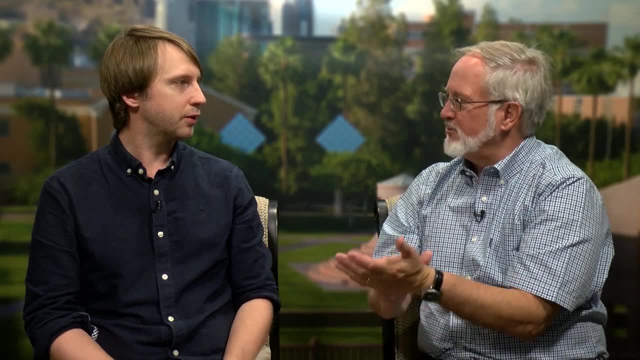 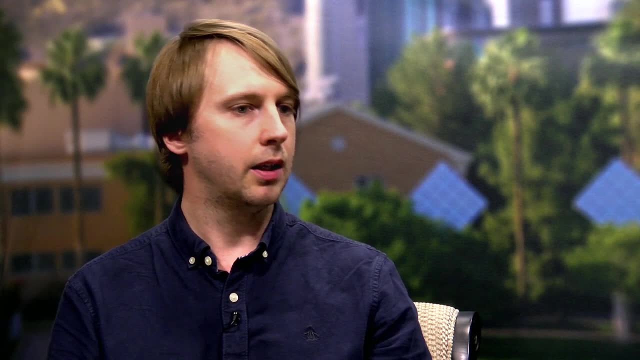 fighting them when they're in a biofilm, and that's the big advantage: They protect themselves. So on a heart valve, for instance, it's a desperately problem. The antibiotics can't get at them, That's right. That's right. They form multiple layers of cells. The antibiotics can penetrate. to some extent, but it's the cells on the outside that will tend to suffer. The cells on the inside aren't growing, and that's a big problem for antibiotics. Antibiotics target growing cells predominantly, So biofilms make everything sluggish and slow down. 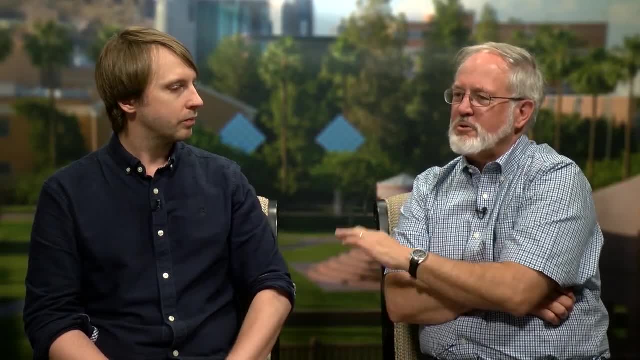 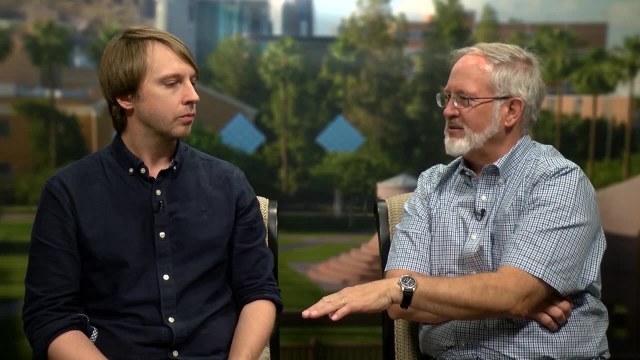 Mm-hmm, And that makes them a real nemesis. I was a part of a group a while back that was trying to figure out ways of interfering with the cooperative tendencies of bacteria so as to break down the biofilm so the antibiotics could get in. Has anything come of that? 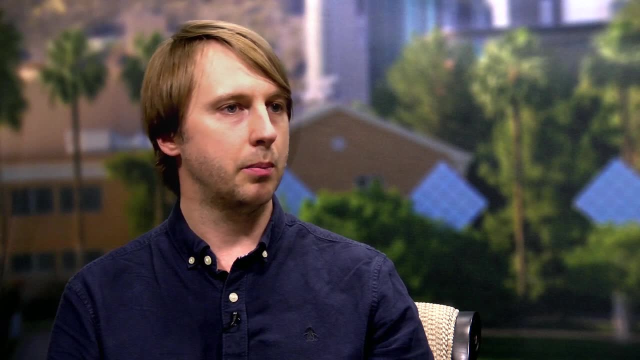 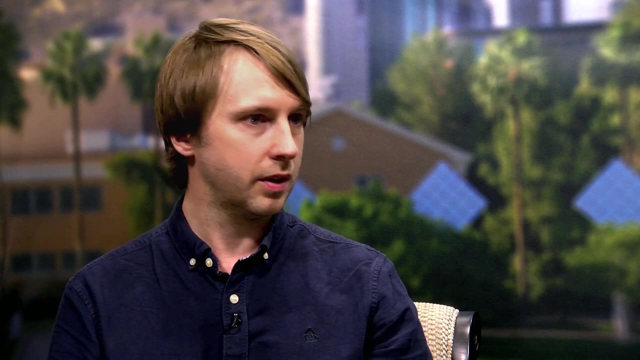 I mean we don'tthere's no drugs yet on the market, but I mean I'm involved with projects where we're doing that and it does seem to work. Is that right? Yeah, So we can indeed inhibit biofilm, so the adhesion that holds the cells together. 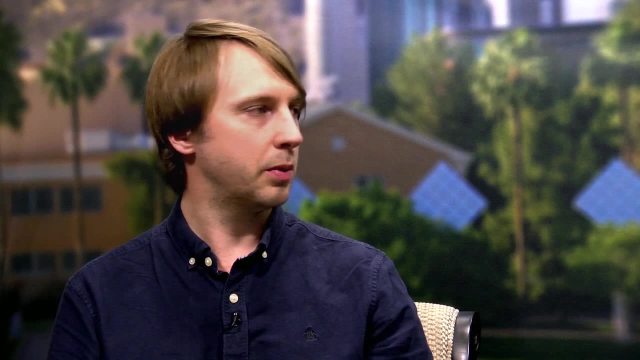 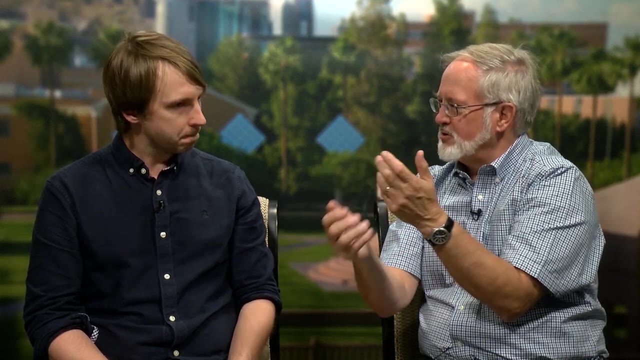 And in doing so we can disrupt biofilms in a way that wouldn't be possible with just simple antibiotics. So do you disrupt the proteins that hold them together, or do you also attack the signaling molecules that they use to tell each other what to do? 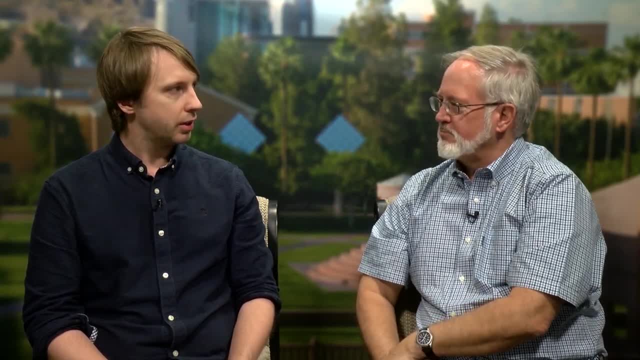 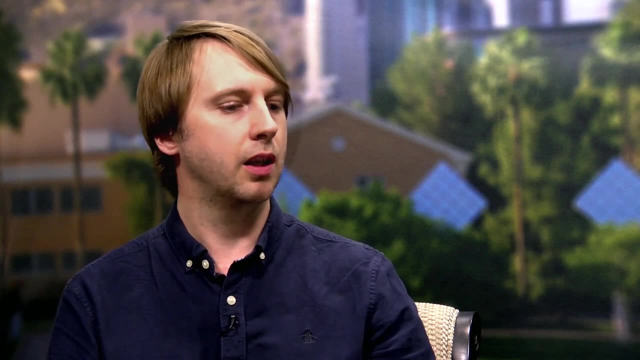 So certainly some people are interfering with the way the bacteria communicate with each other. So theybacteria displaysorry coordinated responses under what's often called quorum sensing, which allows them to do everything in synchrony. What's quorum sensing mean? 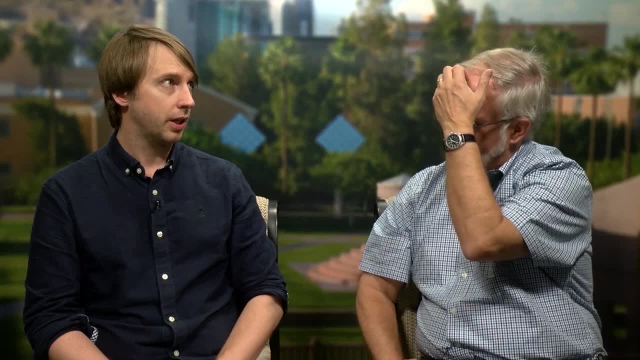 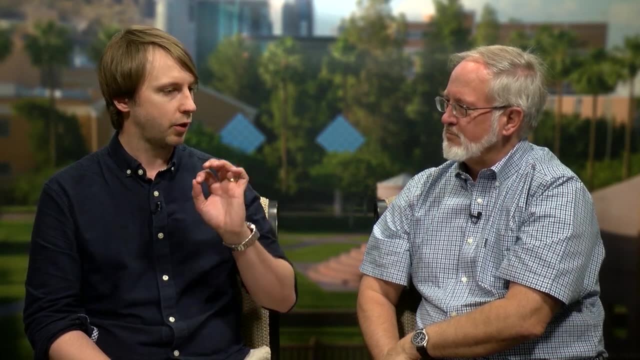 Yeah, So that's a good question. So quorum sensing is basically a trick, a clever trick, that bacteria have to assess the density of the cells in their environment, And the way they do that is they throw out small, inexpensive molecules into the environment If there's. 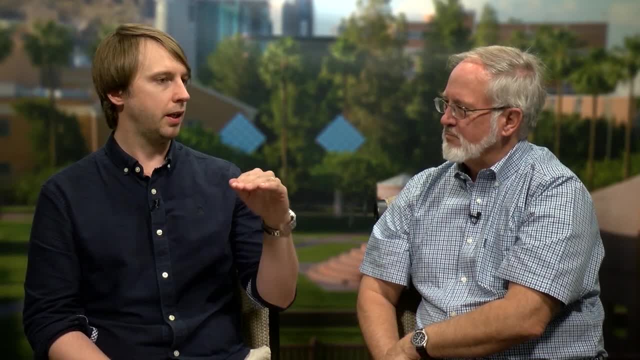 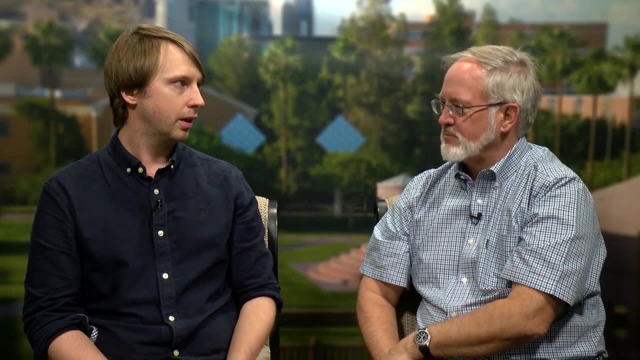 a lot of cells around, then the concentration of those molecules will be high and they can detect that. So there's enough of us. Let's act as a group Exactly, And it'sagain it's very important in infection. So things like MRSA, this sort, 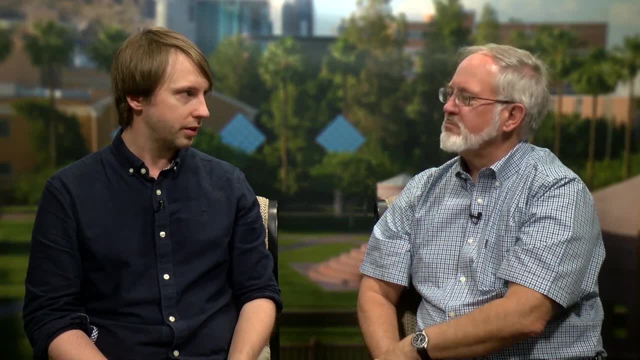 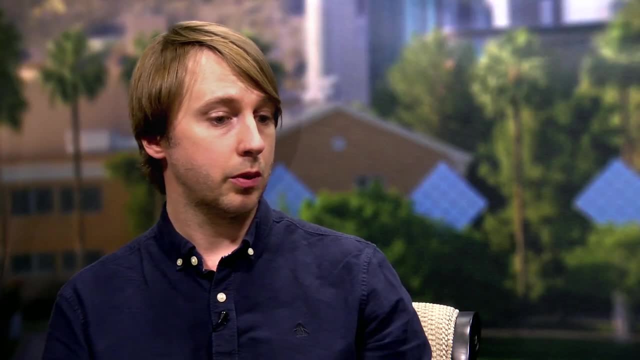 of problematic. What's that? So that's Methicillin resistance. Staph aureus? Yeah, exactly, Staphylococcus aureus. So this is one of the sort of superbugs people worry about in hospitals. So the way that that evades our immune systemwell. 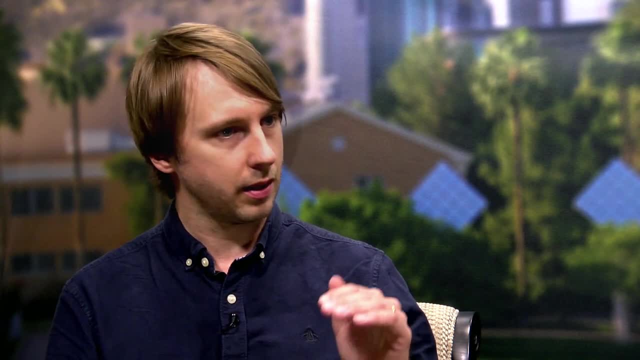 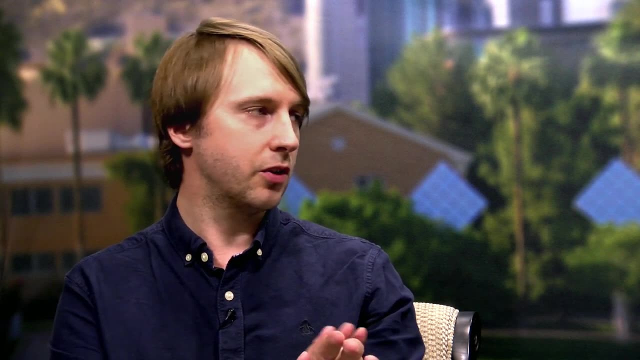 our immune system, at least in part, is by coming in quietly. So basically it'll go through a breach in the skin or somewhere, find its way to a bone surface, form a biofilm, and in all this time it's not really doing that much. 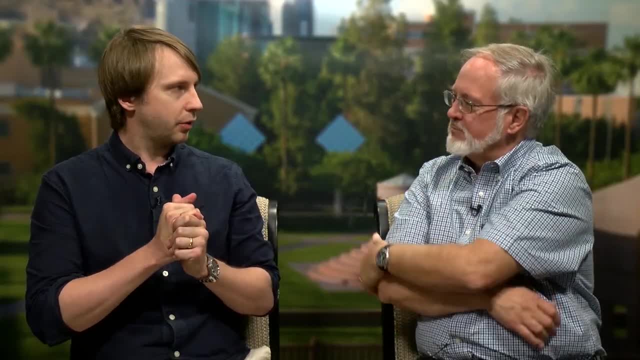 So you don't even know you have an infection maybe. Well, the immune system exactly is under the radar, But then at some point, when it has enough cells and the quorum sensing is activated, then it engages its attack. 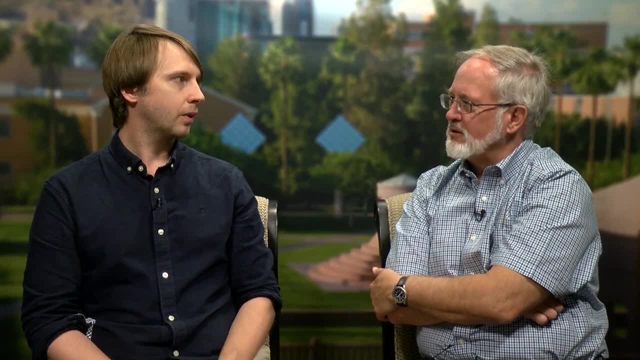 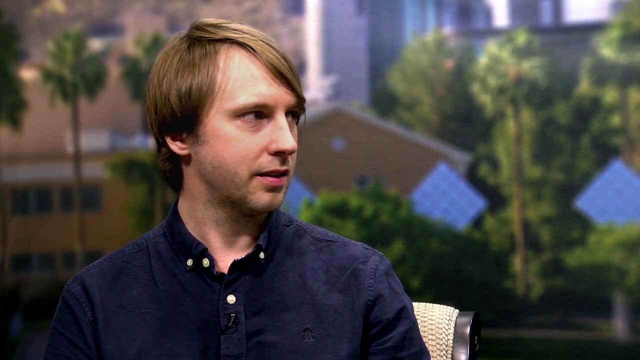 So if we could disrupt that quorum sensing, that might be a great thing, And it is something that people are trying to do. The big challenge is having the drug there at the time, You know, at the right time in the right place, And that can be challenging because 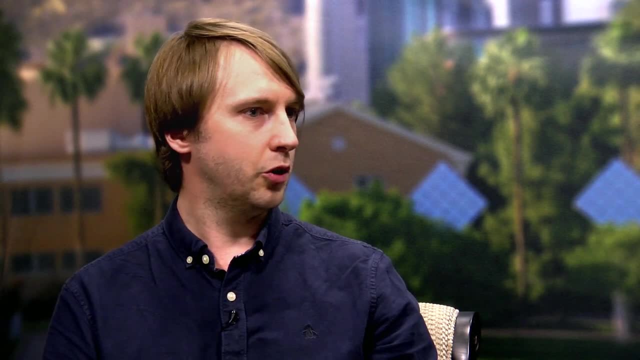 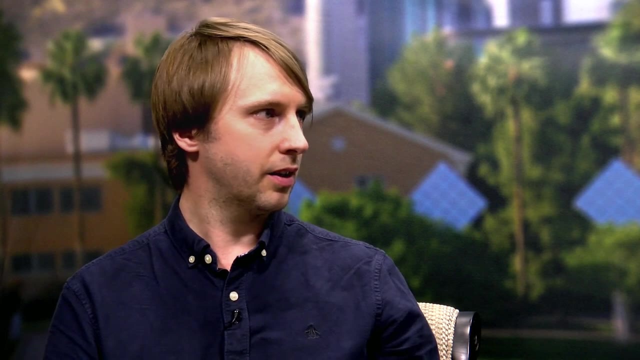 it's a specific, you know, stage in the infection process, And normally we treat diseases only once we see symptoms. So the problem is prophylaxis, as it's called. You'd have toto make this work well. the concern is you'd have to keep people on drugs ahead of time, which sometimes 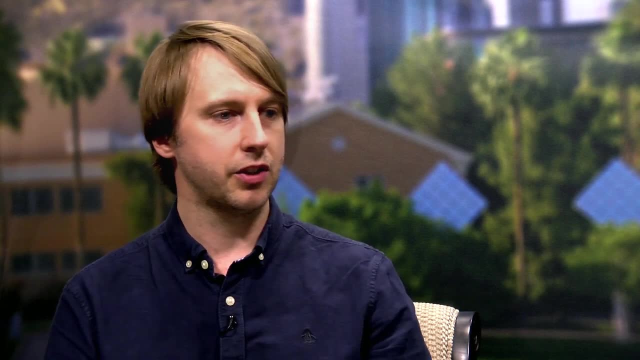 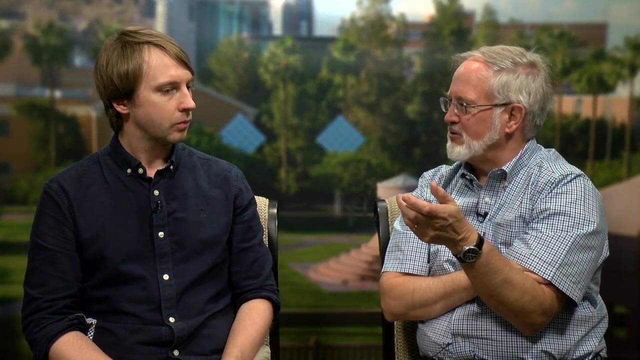 is appropriate For surgery or something sometimes, But it's a challenge Maybe. yeah, But it's a challenge. So do all microbial biofilms have just one species of bacteria or there's some way multiple different species can get together to do things? 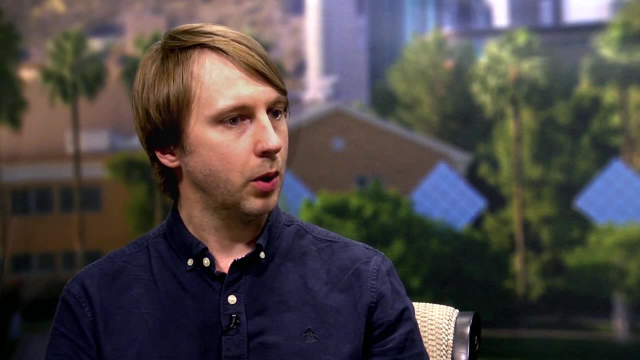 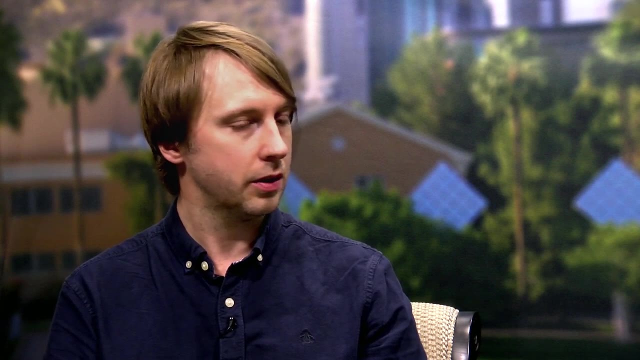 Well, certainly a lot of biofilms. It's in form with multiple species present And indeed polymicrobial disease, as it's called, is a real thing, and it's where you have an infection, where there's multiple strains present And there's 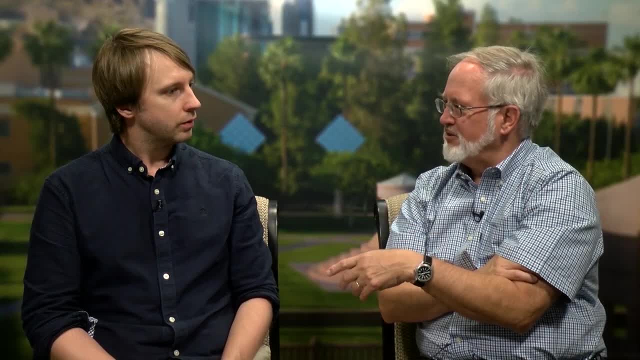 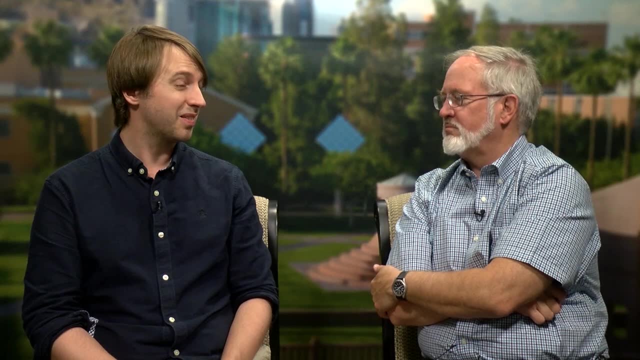 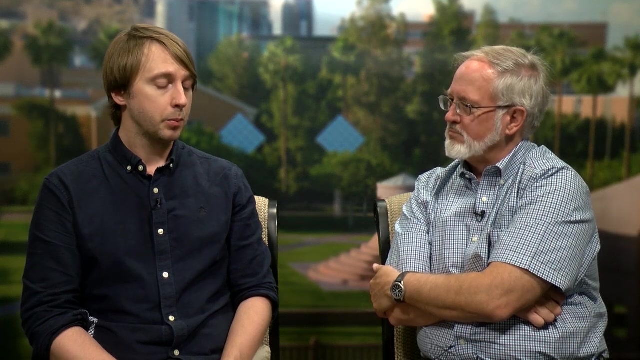 So that's quite different from our standard medical thing of find out what bug it is, Exactly exactly. This is, you know, yes, a major problem for diagnosing and treating disease if there's multiple different species contributing to a particular disease trait. But yeah. so I might add something: Are they all probably gram-negative, or will you get diversity? No, you can have real diversity. That makes it hard. It can do. yes, I mean, broad-spectrum antibiotics are one option. 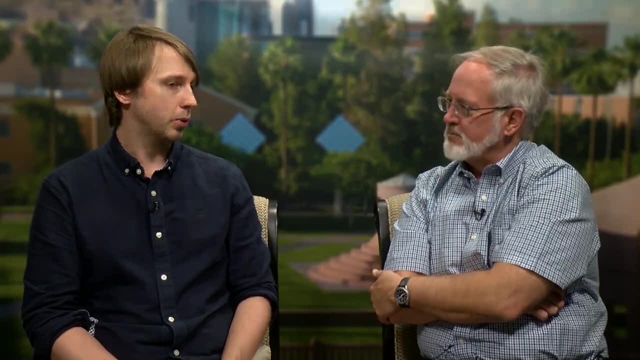 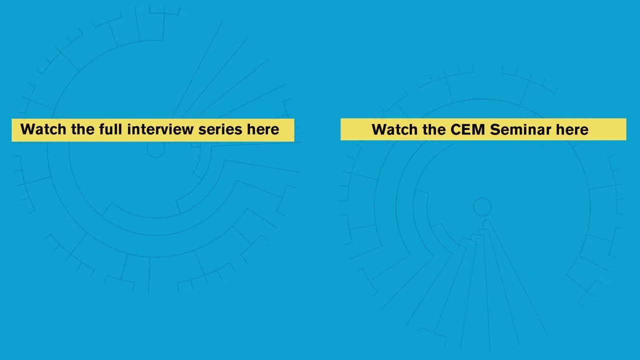 But certainly understanding what these guys are doing and how they're there is important You. 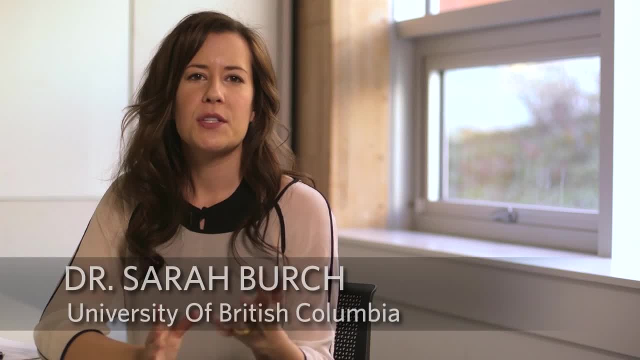 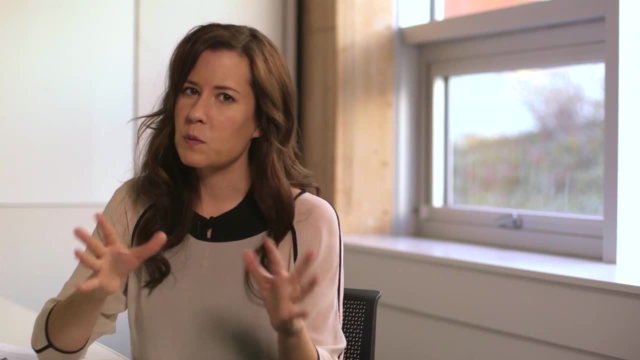 In lecture 2, we'll explore one set of strategies that can be used to help mitigate climate change – demand-side strategies. In the lecture that follows, we'll explore the challenge of renewable energy, which is the core element of supply-side strategies.